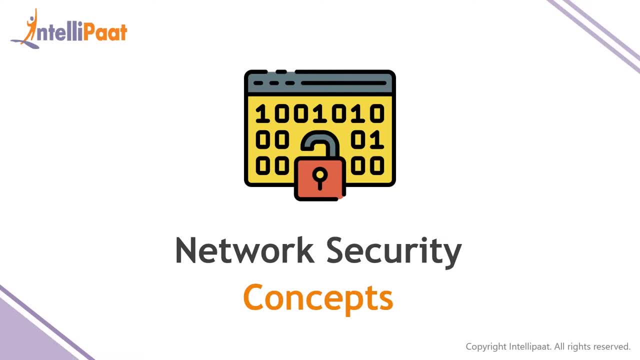 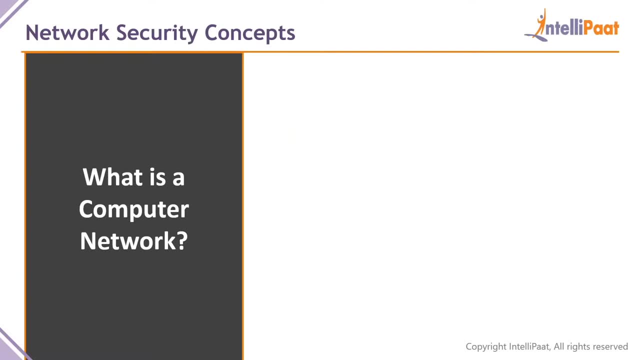 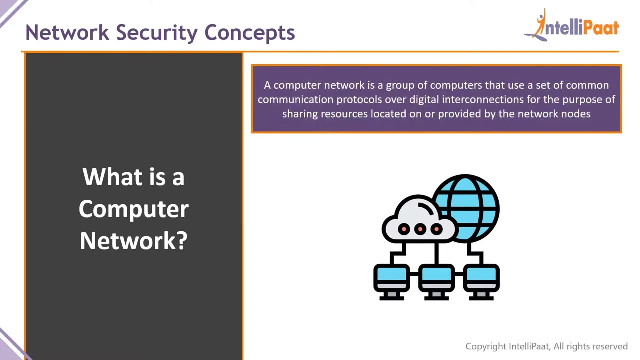 So network security is quite a broad field of study, Right? So we need to understand, firstly, what is a computer network? Right? So we are protecting something, We need to understand what we are protecting. So a computer network essentially is a group of computers that use a set of common communication protocols over digital interconnections for the purpose of sharing resources located on or provided by the network nodes. Right? 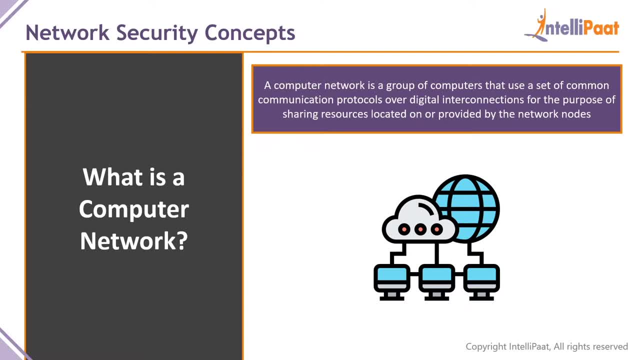 So imagine you have a lot of computers in a particular office space together. Right, You take LAN wires, you connect all of them to a server, Right? So what will happen is, essentially, all of those computers can share their resources, can share data files, can share other things as well, such as processor resources, server resources, RAM and whatnot, Right? So when you connect all of them together, you're creating a network of computers. So that is called a computer network, Right? 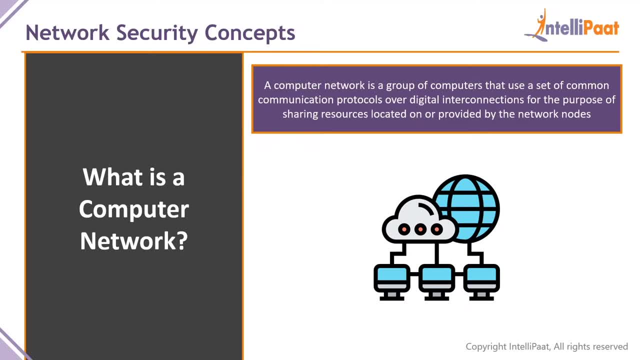 So now that we understand what a computer network is, we need to understand network security as well. So network security essentially is defined as the implementation of technologies, processes and protocols designed to safeguard an individual's or organization's communication and communication Right. So naturally, if you have a computer network, there's a possibility of the data being circulated around that network being leaked or some other interruption that happens within the network And you need to prevent that Right. So you implement these protocols, these technologies which come under network security Right. So this is an entire field that deals with this particular issue. 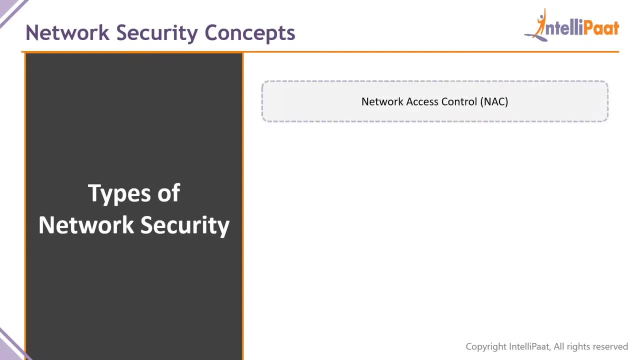 So there are types of network security. So, firstly, there's network security, There's network access control or the NAC. So network access controls is exactly what it is named. It's basically to prevent other users from getting into the network who don't have the proper certificates or policies, Right? So if your network has a policy for not allowing strangers to basically visit your network without the proper authority, So you're implementing network access control. It is used to implement endpoint security, Right? 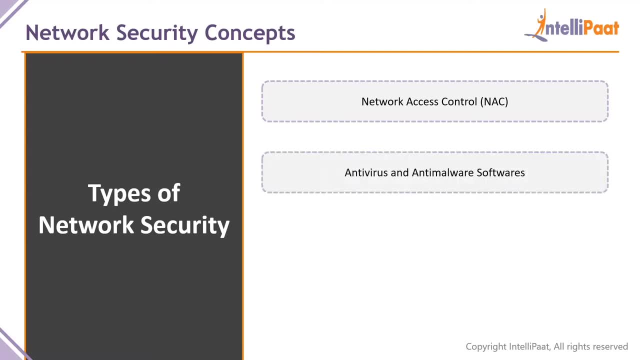 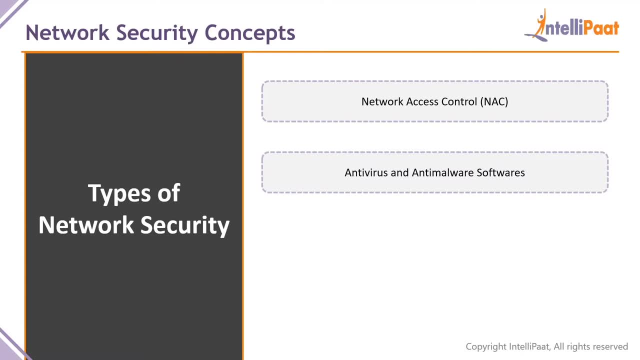 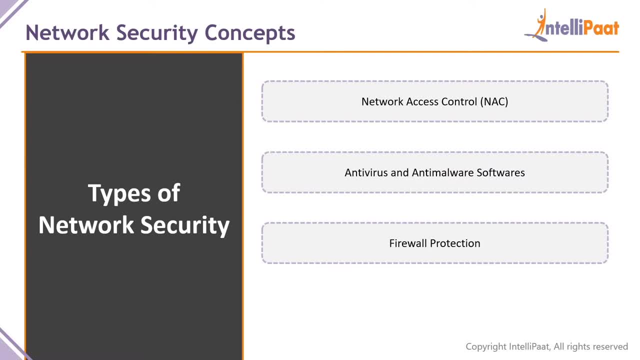 reports that are open for application interactions with the Internet, with the network, the rest of the network. you can go ahead and basically create some rules that restrict your private network or restrict you from basically being exposed to the public network as well, from mostly where you're concerned is inbound activity, So basically any external network, any external server, any external website or application that tries to ping your network. 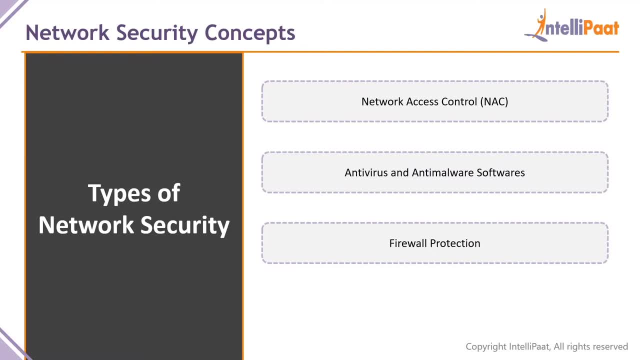 bring your particular node and try to get some information out of your particular node or try to install something onto your particular node. if your inbound rules of your firewall do not allow anything other than the particular things that you actually allow, your firewall will effectively stop that. so that is what the firewall essentially does. it also does the same for outbound activity. 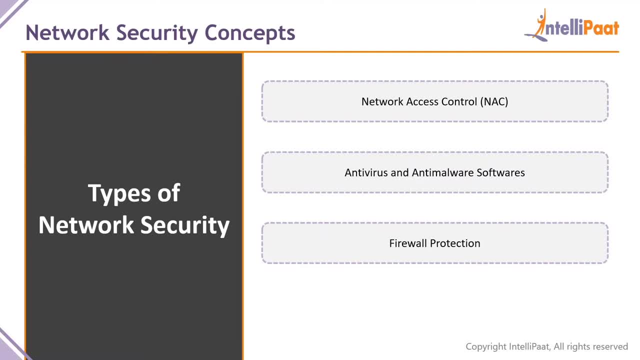 so basically, if you're restricting your employees from basically accessing anything outside of their office work, or your school students from accessing anything outside of their study material, you can impose that onto the firewall as well. then we have a virtual private networks now. virtual private networks essentially help people to hide their original identity on 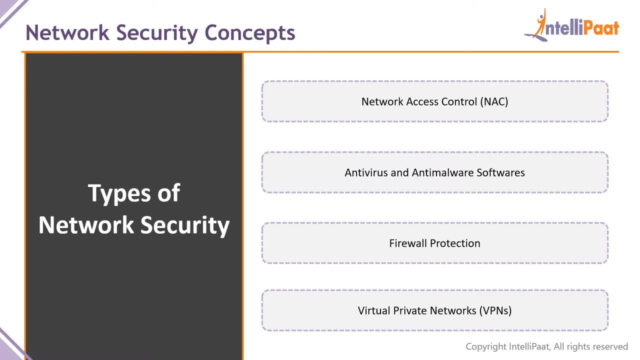 a network. so basically means that they tunnel in a network and basically come through different nodes attached to different nodes and basically mask their original ip and their original mac address and get access to the network without actually having to reveal any information about them. this also ensures a end-to-end encrypted setup, so that means that anybody trying to access the 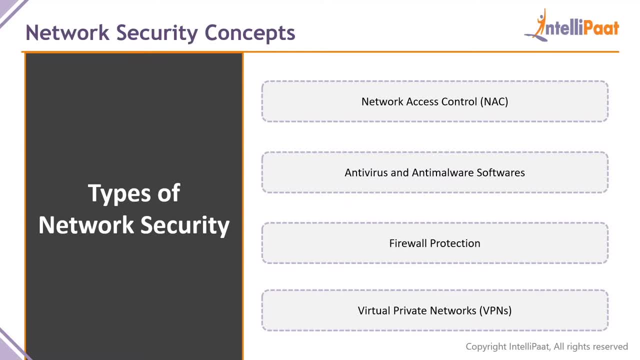 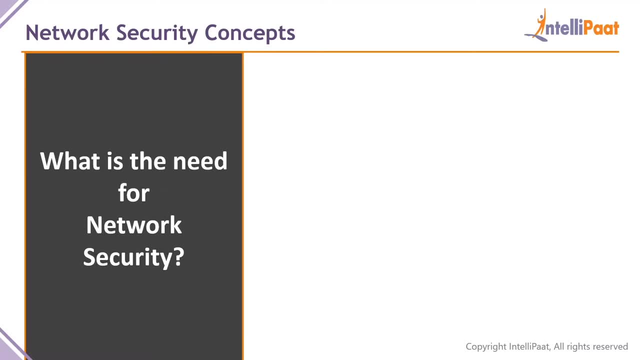 information being shared to and fro outside of a vpn tunnel cannot actually access it. so what is the need for a network security? so the need for network security is quite prominent. so if you're a sender and you have a message that you want to send to your 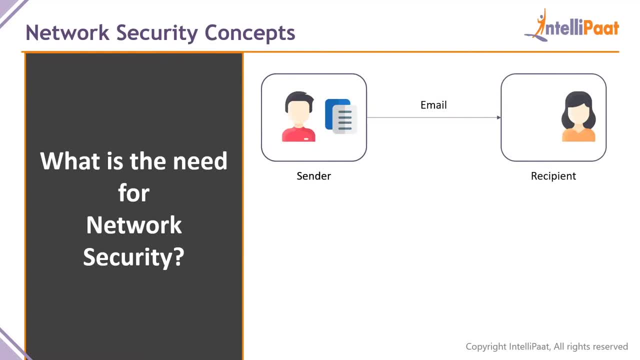 receiver, right the recipient, and you're sending that message through email. so, naturally, your first course of action would be to simply send the email. this is what you think the email diagram looks like. you simply send it to the recipient, but there's a problem if there's an intruder and your network is. 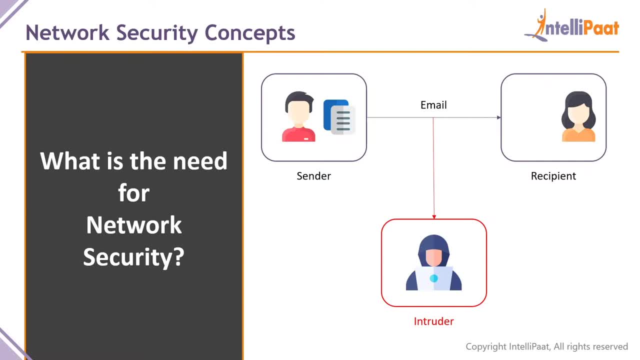 basically compromised. if somebody else access has access to that network, right, and they can basically track your email, so they would get the email as well. now, if this email contains sensitive company relevant information, this could be extremely harmful for your organization, so you don't want that. so, uh, your intruder is able to read your data. you do not want that, so this: 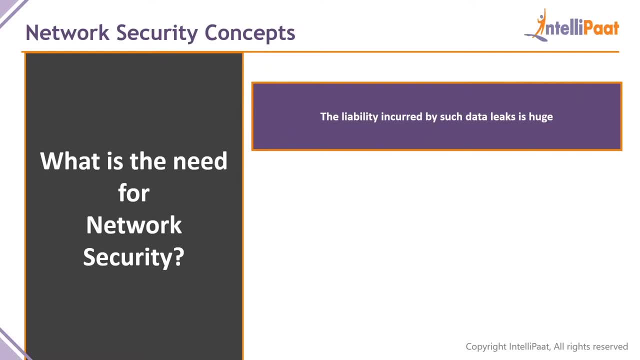 liability. uh, could be small, it could not mean anything if somebody else gets access to their data, or it could be really huge as well. right, so this could lead to monetary losses. if the competitor gets access to your sales information, your customer information, your strategies, this could lead to monetary losses if somebody basically files a case on you for basically allowing their 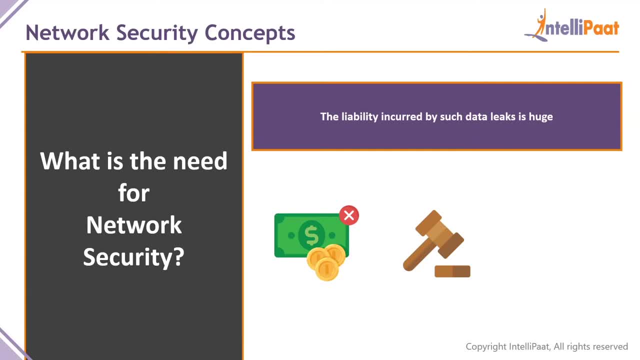 data to be leaked to the public or to the hacker. the court can also file- a court can also rule against you in that regard- and then you'll have to pay damages in monetary revenue. so that could also lead to loss and at the end of the day, it leads to employee and customer dissatisfaction. 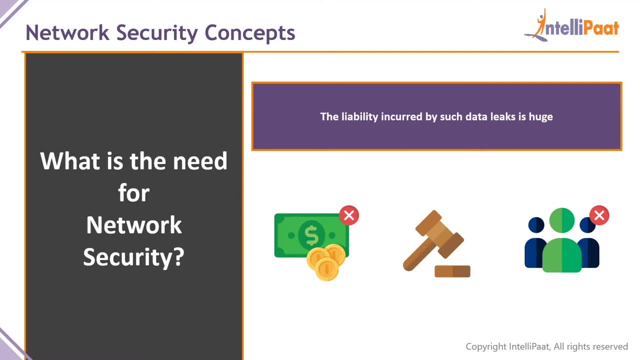 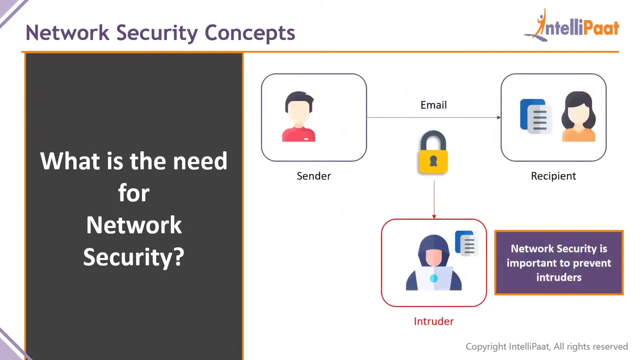 and distrust in your organization if your organization does not have network security and intruders and hackers are able to get the data right. so all of this is something that you entirely don't want, and that is why you need a network security- almost certainly, so what you 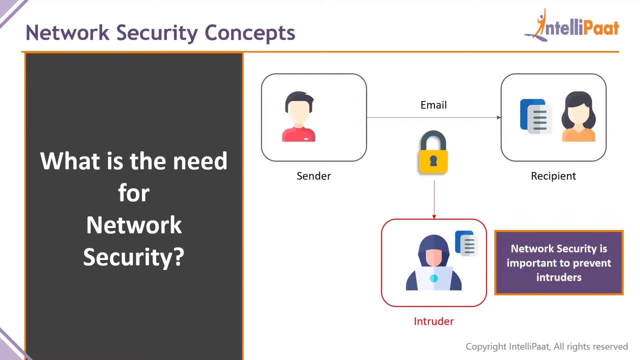 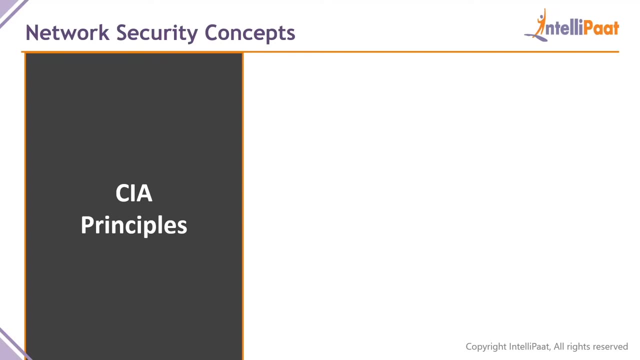 will do is we will basically lock your line of connection between the sender and recipient so that intruders cannot access it. so this lock, essentially this metaphorical lock, is what network security is. so let's talk about the CIA principles. this is not to be confused with the intelligence. 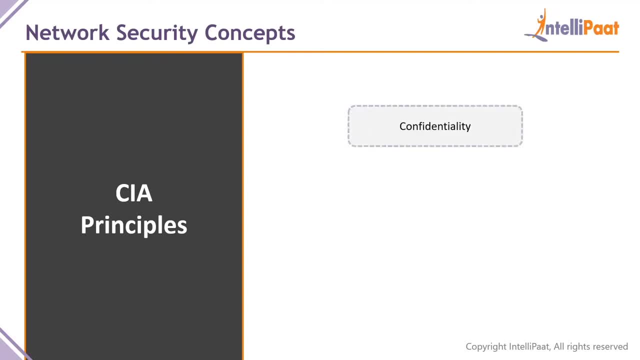 agency. these CIA principles basically means confidentiality, that means secrecy. so the data that is being transferred to and through, or the data that is being contained on the network should remain confidential if needed, right. so that is the first principle of network security. the second is integrity. so the data should be whole, the data shouldn't be less. 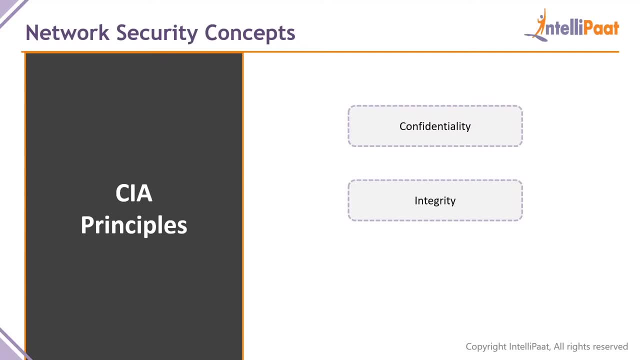 than less than what it was, and it shouldn't be more than what it was. the data should be exactly identical to the original data that was there. nobody should have been able to manipulate it. the data should not have been lost. to verify this, we use checksums. to verify this, we use a lot of. 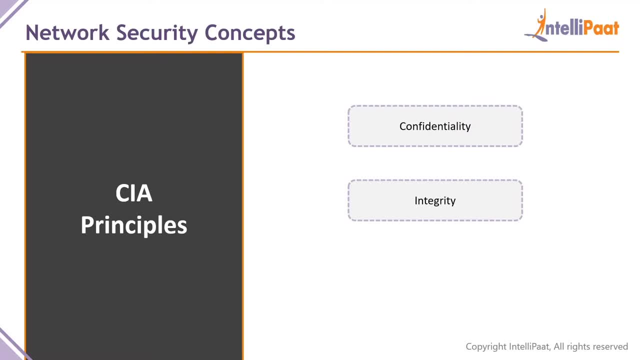 other methods as well to check the sender, to check the, basically the contents of the file, whether they are the same or not. so this is integrity. and, finally, we have availability, so the data that has to be accessed should be available to the intended recipients at all times, at a very short notice. so this data 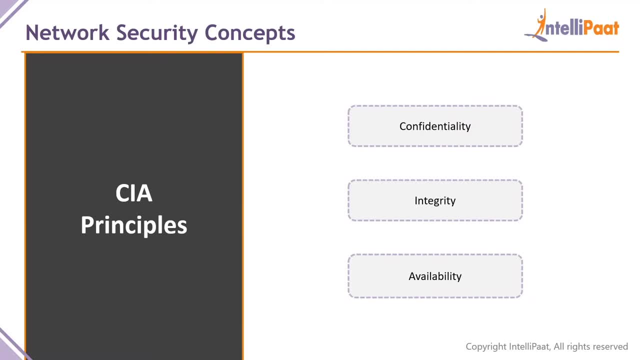 obviously needs to be accessed by the relevant people for the organization or the business to continue, so the data should be available as well. so, aside from confidentiality and integrity, you cannot keep this data stored away securely forever. you need the data to be available as well, on demand. 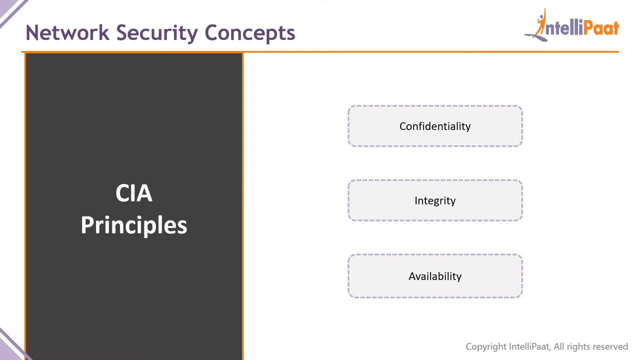 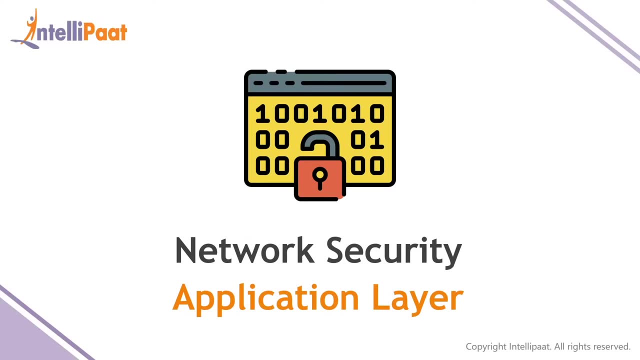 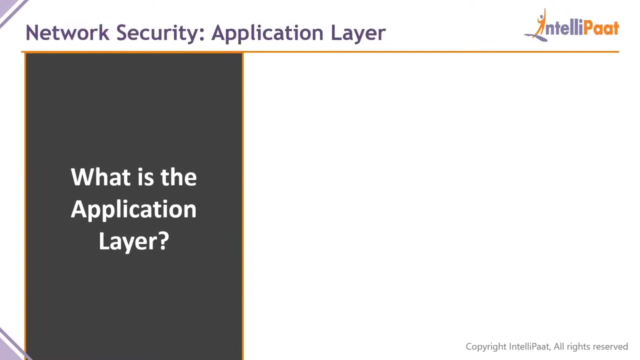 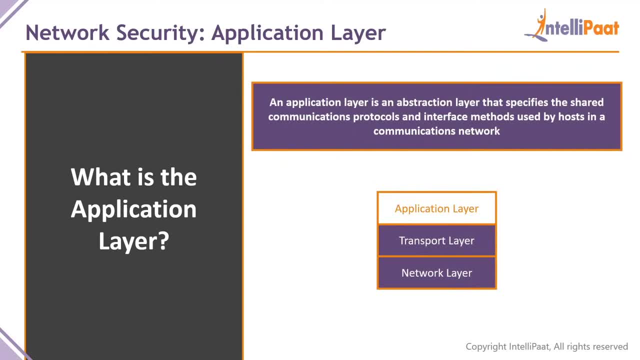 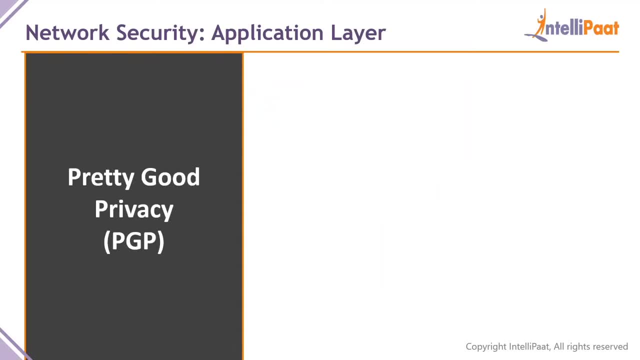 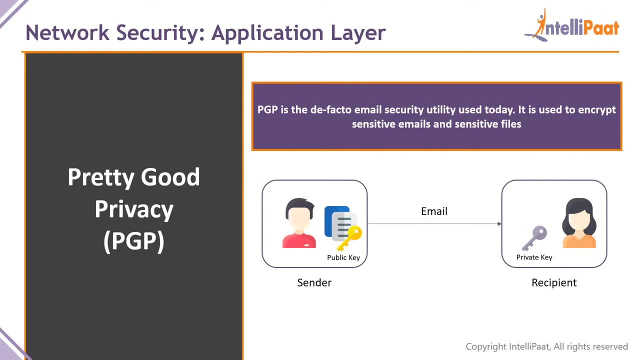 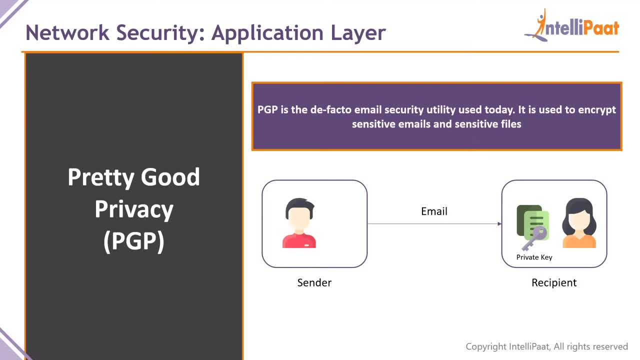 not have access to it. nobody else has access to the private key. if the public key leaks, it does not matter, because the private key is needed to decipher the message that has been sent. so then the recipient will decipher the message and then the recipient will have access to the actual. 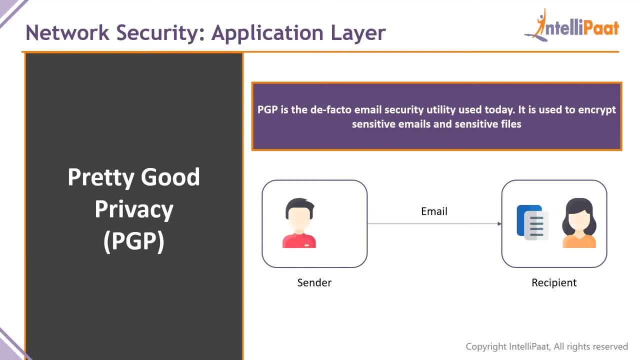 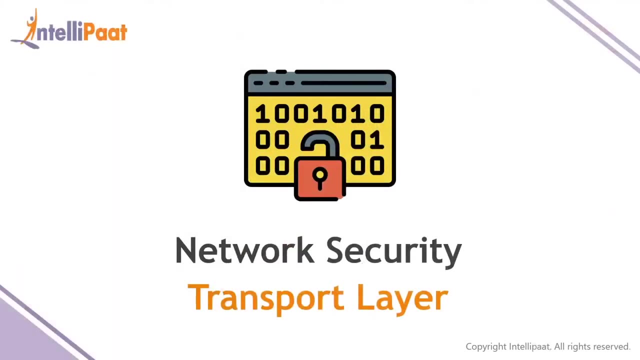 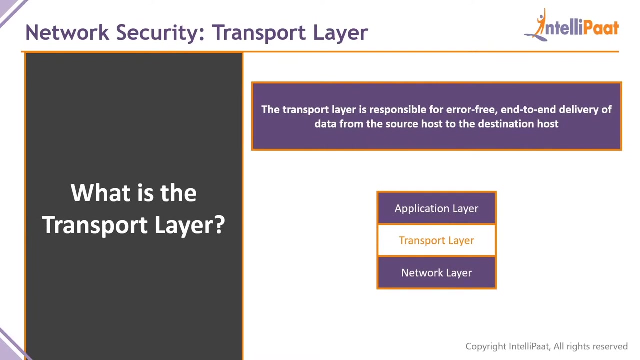 intended message. so this is how pgp works it is. it can work on symmetric security measures as well, but this was an example of an asymmetric email authentication system. next up we have the network security transport layer. now transport layer is the second layer effectively in the diagram. so the transport layer is responsible for error-free end-to-end delivery. 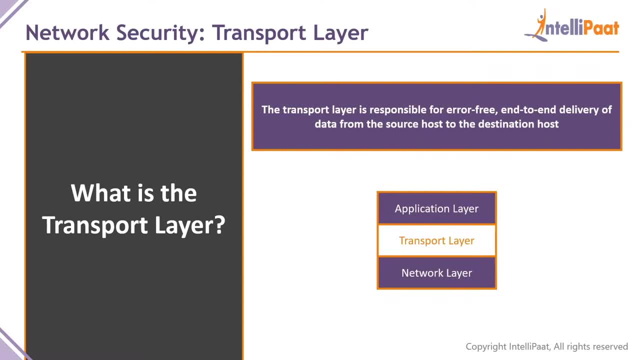 of data from the source to the destination host. so this basically means the transport layer primarily deals with data integrity, because it wants the data to be error-free. right, it's not particularly responsible for the security of the data, so this is an example of an asymmetric security aspect of things. but it wants the second principle of the cia principles, called integrity. 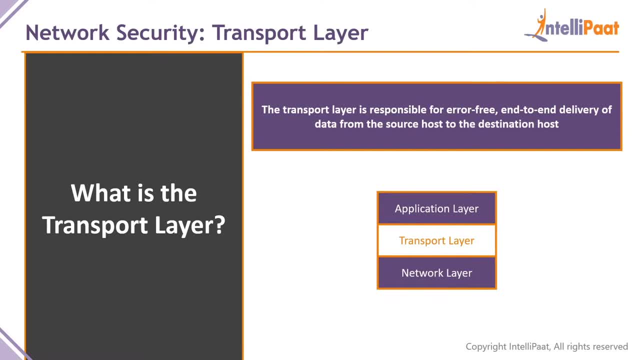 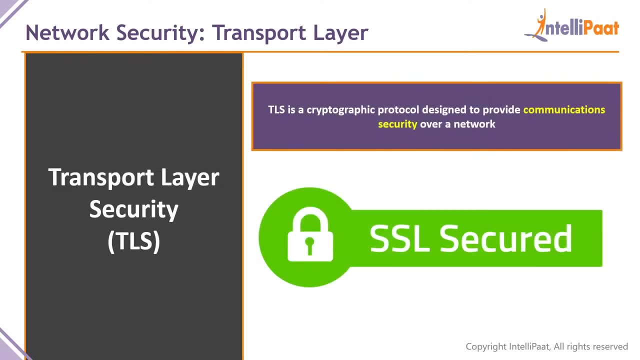 right. so that is what the transport layer essentially deals with. so let us see one of the examples of the transport layer called the secure socket layer. the secure socket layer is now transformed into the transport layer security, which is the successor to the ssl protocol, essentially so. the tls is used today, so tls is used today. so tls is used today. so tls is used today. 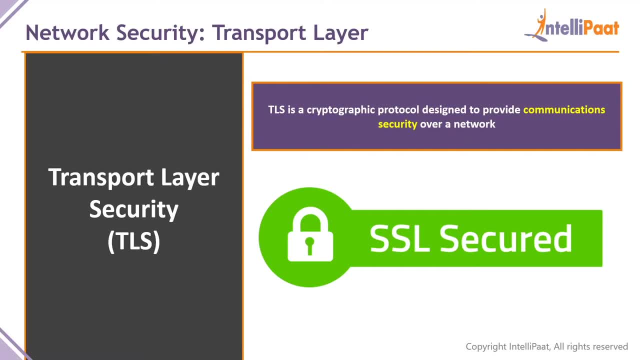 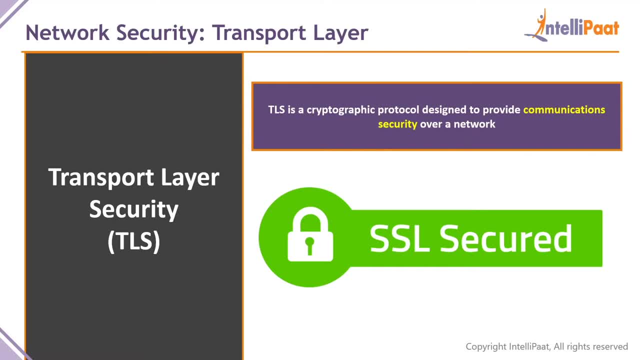 any web application that you're trying to access over the internet essentially will have an ssl security certificate. if they don't have that certificate, your web browser will automatically tell you that this website is not secure and it is not recommended to provide security security to proceed forward. i'm sure you must have seen that whenever you try to log into a website, some 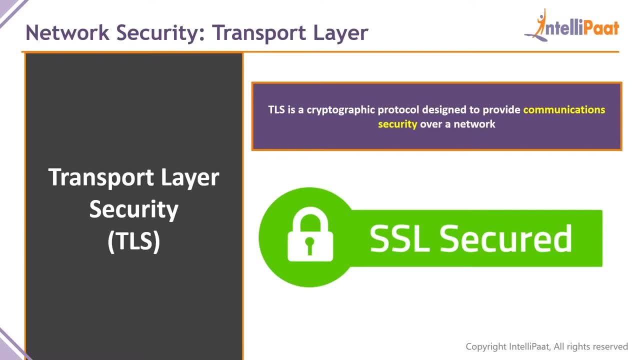 website- uh, you might come across once that has this message on google chrome, which is, which says that the connection is not private, uh, because it does not have an ssl security certificate, right? so tls is essentially that cryptographic, cryptographic protocol that ensures that the website has ssl certificate, right? so this is a communication. this is used to provide communication security. 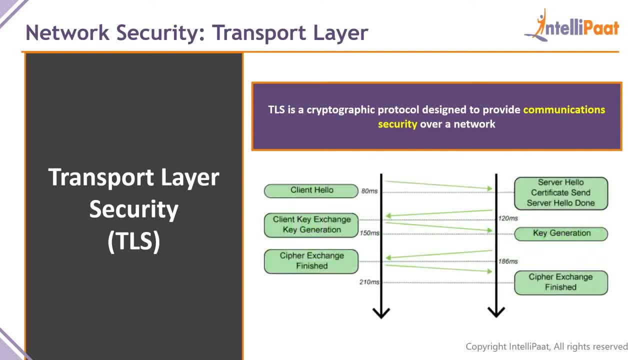 communication security over a network. so let us look at the diagrammatic representation of this. so the client, which means you, who is trying to access the website, will send a hello message, right, the server will send a hello message and then the server will then send the certificate. 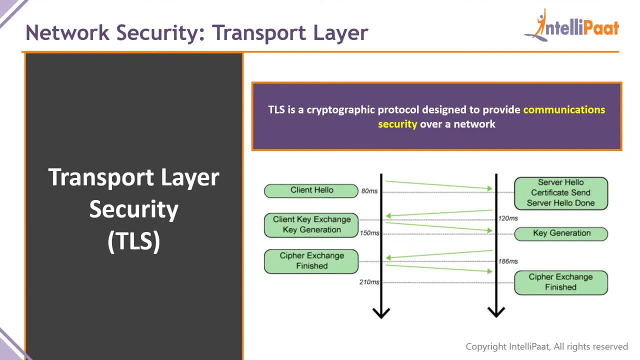 to your web browser the ssl certificate that it has. your web browser will then authenticate that certificate, essentially by checking in the database. if the certificate actually exists, is it genuine. when the certificate has been authenticated, the server hello has been done. the client will then provide the key exchange to create an end-to-end encrypted transmission. 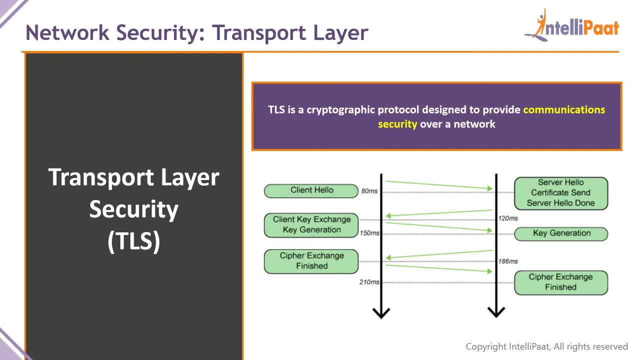 between the client and the website in question right, so the client will essentially start the key exchange process. the key generation will happen on the client's end, as well as the websites, and, and once the keys have been exchanged, the cipher exchange has been finished on both ends. 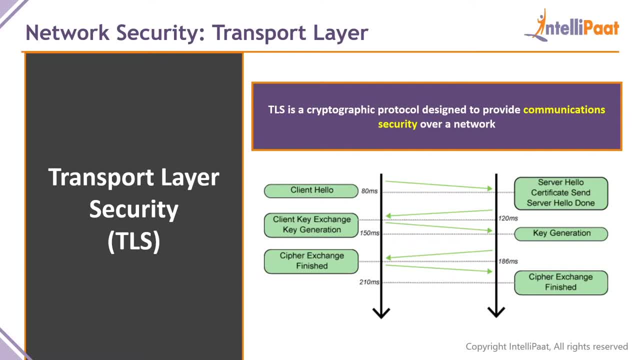 then the secure protocol has been established, because all messages, all security communications, from then on will be encrypted and they will not be decipherable by any outside attacker or intruder. so, essentially, all the interactions that you have from within the website are encrypted in nature and nobody else can have access to it, unless, of course, your isp is tracking you, unless 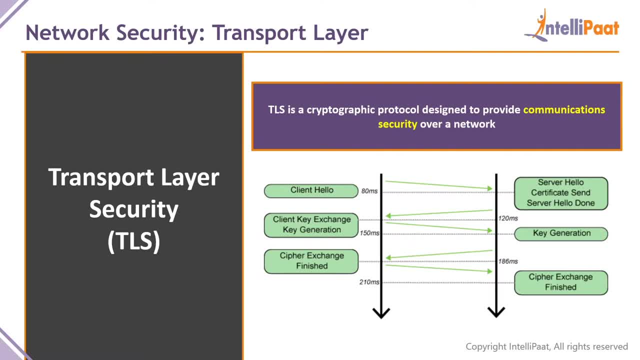 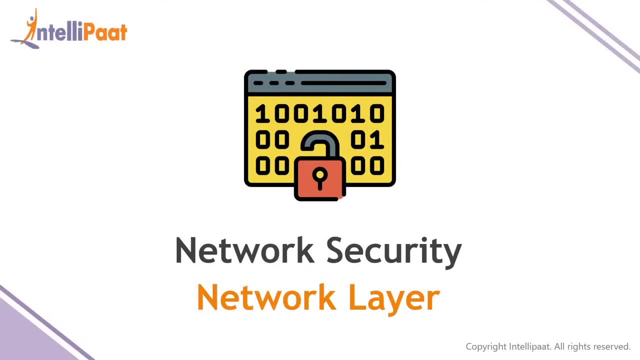 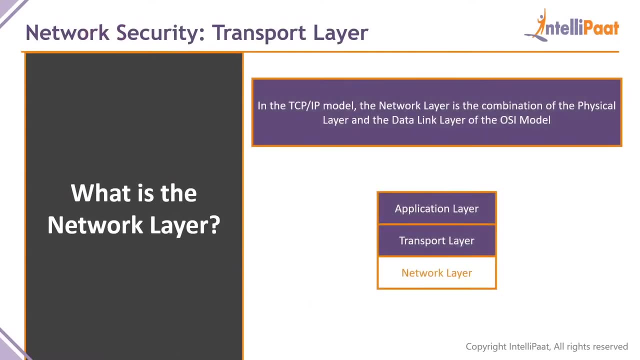 of course your employers are tracking you. that is a different case because they are tracking you from the client's end. they're not tracking you from the website's end. so let's look at a network layer, the last layer in this particular tutorial. so the network layer essentially deals- uh, in the tcp ip model at least the network layer. 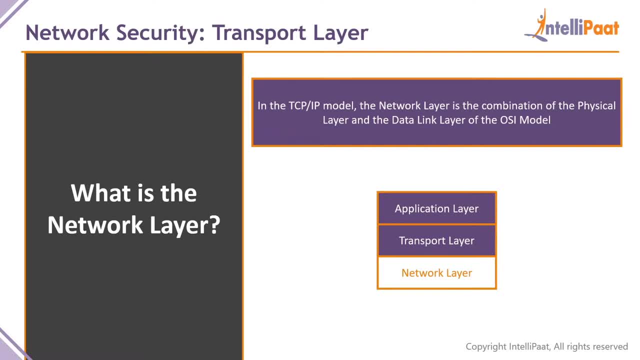 deals with the combination of the physical layer and the data link layer of the osi model. now, here the physical layer refers to the actual physical connection between your host and the recipient host. that is the actual physical connection, And the data link layer essentially refers to the data synchronization layer, where it is ensured that the data that you're sending is actually sent to the receptive layer in the receptive host or the receptive node in a particular order. 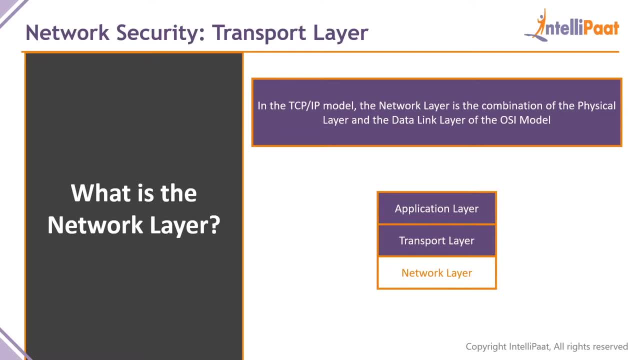 So both of those functionalities have been combined in the TCP IP model and it is called the network layer, So it is responsible for mapping IPs into physical addresses. So in a particular network you have your IP addresses, your local IP addresses, and then you have the MAC addresses, which are also called the physical addresses. 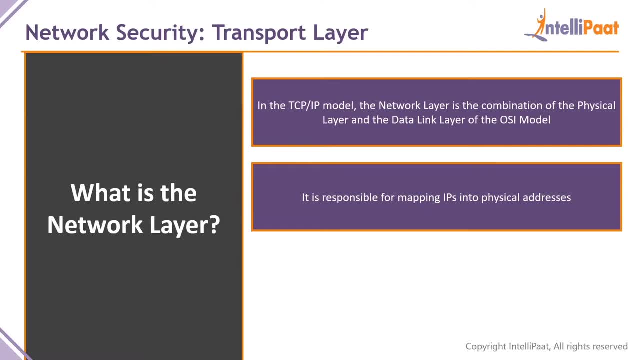 So in any particular network, once the pinging has been done, once the network has been mapped up, the IPs are mapped to their devices' respective MAC addresses. So whenever you're trying to send a packet over a network, the network layer ensures that the IPs are mapped to their appropriate physical addresses. 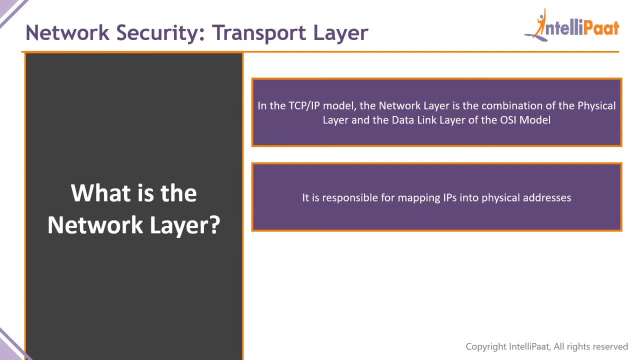 So they're sent to the correct physical address when they're sent Next up. they are mainly responsible for transmitting data between two devices on the same network by encapsulating IP datagrams into frames. So each layer, as we go lower in the network diagram, each layer adds a little something to the packet that is being sent. 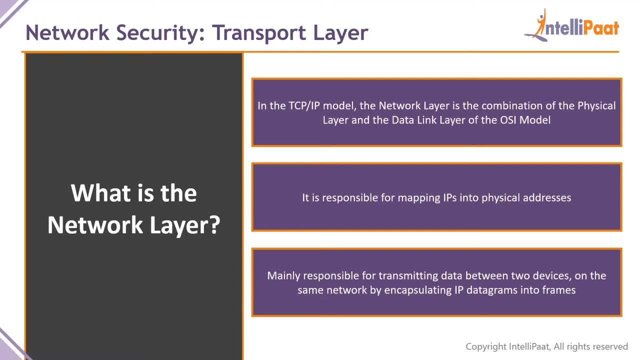 So the application layer will deal with the most minimum amount of information. That information is then wrapped. It is wrapped up in the transport layer and then it is wrapped up further in the network layer into datagrams, essentially. So the datagrams are wrapped up into frames, essentially when they reach the network layer. 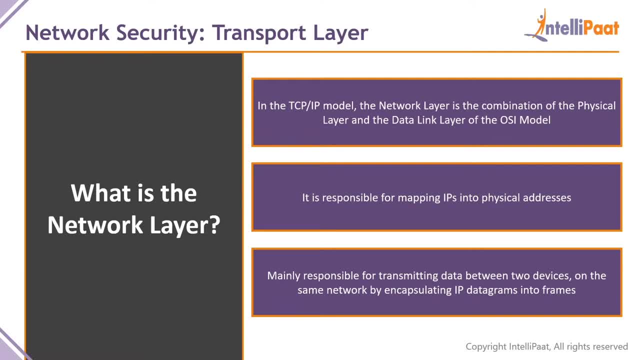 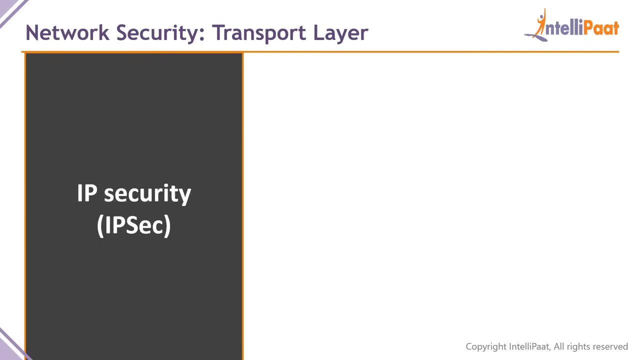 So this is what happens Now: these frames can be sent over the physical layer, the physical connection between these two particular nodes that are transferring data to and through. So, lastly, we will deal with IP security, With IPsec. so this is an example of the transport layer protocol applications. 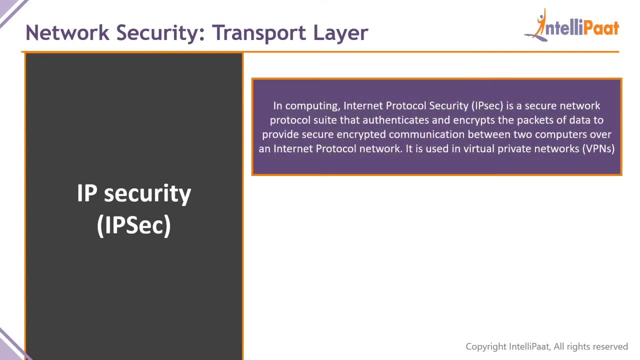 This is called IPsec Now in computing, internet protocol security. IPsec is a secure network protocol suite that authenticates and encrypts the packets of data to provide secure encrypted communication between two computers over a internet protocol network. It is also used in virtual private networks as well: the VPN. 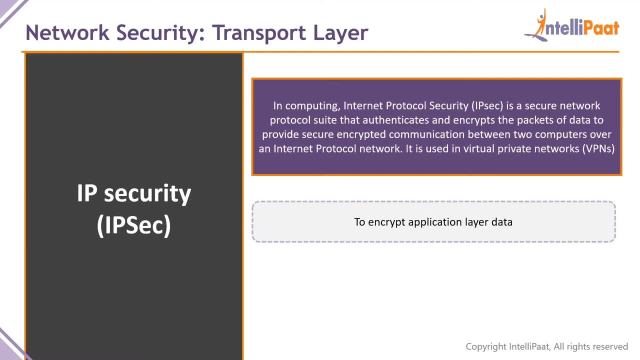 And it is used to encrypt application layer data. So whatever application layer data is being sent to the transport layer, it is used to encrypt that. It is used for router security as well. So you have a lot of routers and switches present within your network to properly route the communications. 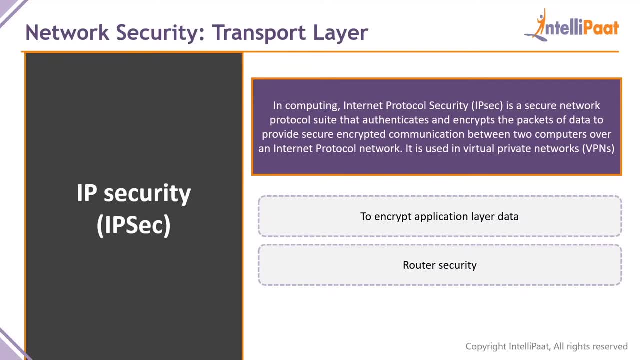 It is used to maintain router security as well by the applying the protocols that it has. and then it is used for authentication purposes, So it adds authentication clauses, So you can send the authentication clauses to your particular data gram and when it reaches the recipient, the recipient checks those authentication clauses to verify whether this particular packet is being sent from the right person or not. 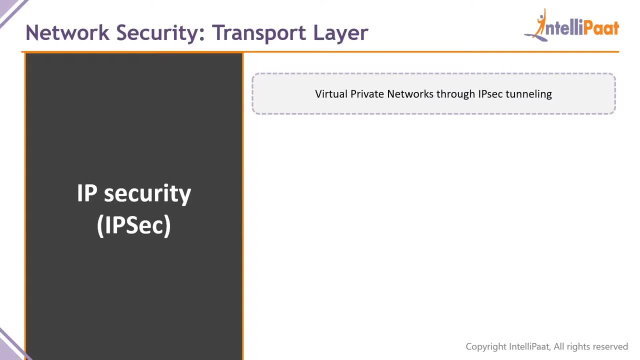 And then virtual private networks through IPsec tunneling. So IPsec also provides tunneling in order for you to create virtual private networks and the tunnels that are required to initiate them And encapsulating security. So, yeah, Yeah, Payload ESP is one of the components of IP security. 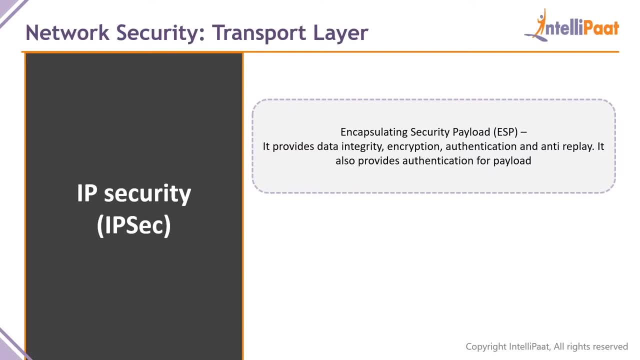 So it provides data encryption, data integrity, authentication and anti-replay. It also provides authentication for payload, So that means that data integrity is ensured with the help of IPsec, which means data that is sent is maintained in its original format. 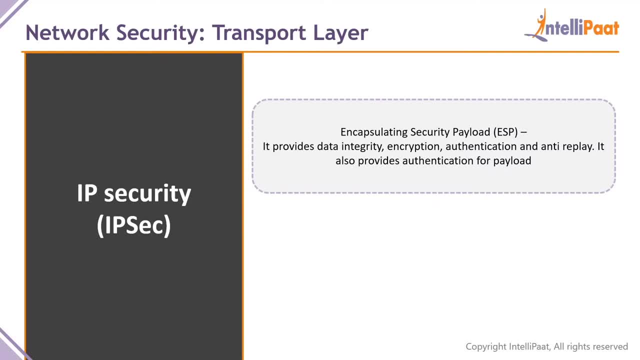 Encryption is an optional feature. You can also implement encryption when you're dealing with encapsulating Security payload- the ESP part of IP security authentication- which means that if you're the intended recipient, then only you can open up the message. You cannot message. 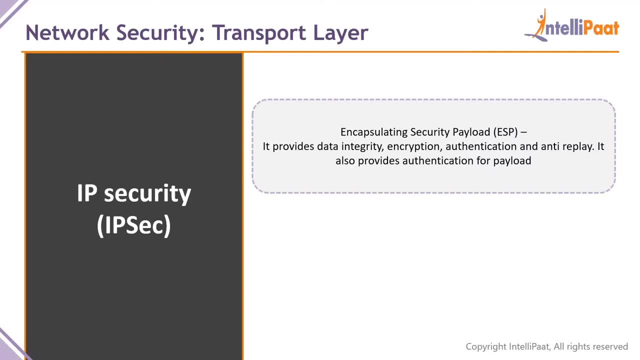 You cannot open the message otherwise. And it is also used to ensure that the message that is being sent is being sent from the right person. and anti-replay, So that means that the message, once seen, gets automatically deleted. Right, So this is also implemented in telemetry. 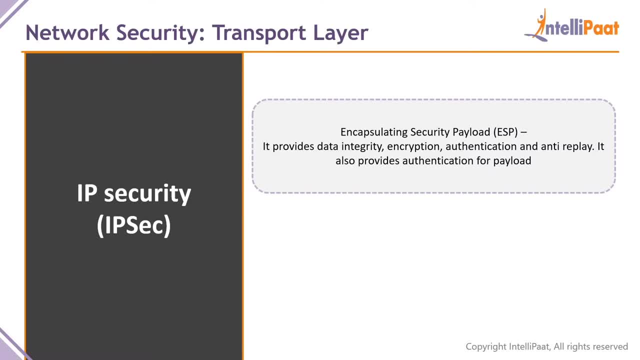 If you're aware of that particular application. So once the message has been seen, it gets automatically deleted so that that message cannot be shared further and the intended recipient can see it, And then the message is done and nobody else can see that message. 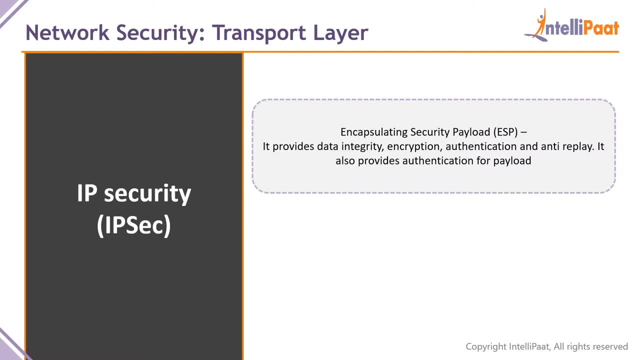 It also provides authentication for payload. So whatever the contents of the message is, that is also authenticated, whether that is correct or not. Authentication header. Now this: This is the second part of IP security. It's also abbreviated as each. 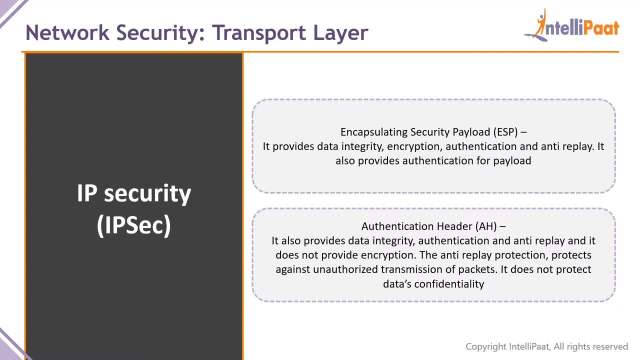 It also provides data integrity, authentication and anti-replay, and it does not provide encryption. So if you don't want to implement encryption in your particular message, then you can go with the authentication header method. The anti-replay protection protects against unauthorized transmission of packets. 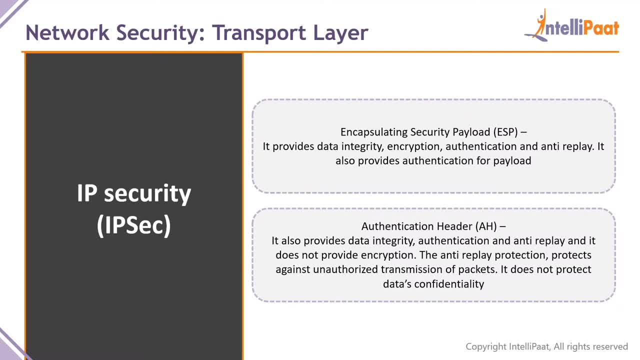 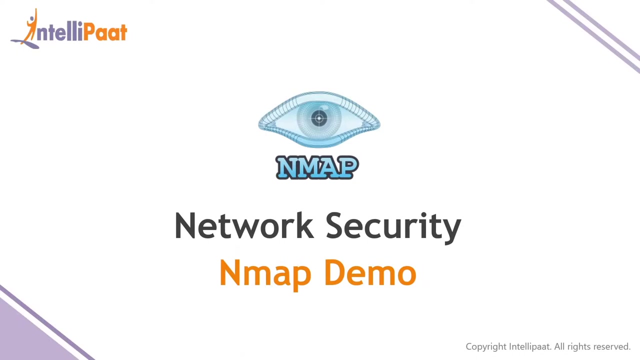 It does not protect our data confidentiality. So that means that since, Uh, this particular protocol does not implement encryption, it cannot ensure data confidentiality. So these are the two aspects of security, IP security. So, uh, we have reached the part where we're going to be implementing the end map demo of network security. 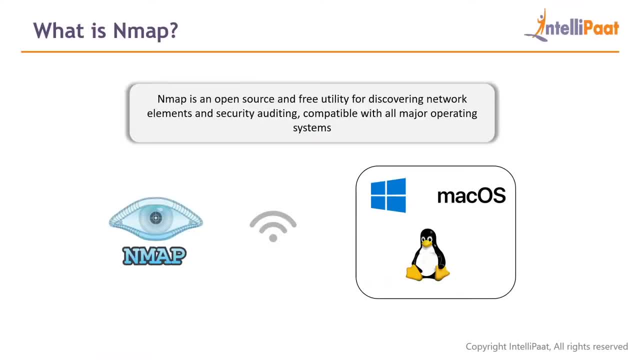 Let us understand what NMAP is first. So NMAP is an open source and free utility for discovering network elements and security auditing. It is compatible with all major operating systems like Windows, Mac OS and Linux, So essentially you can use NMAP to understand the topology of your network. 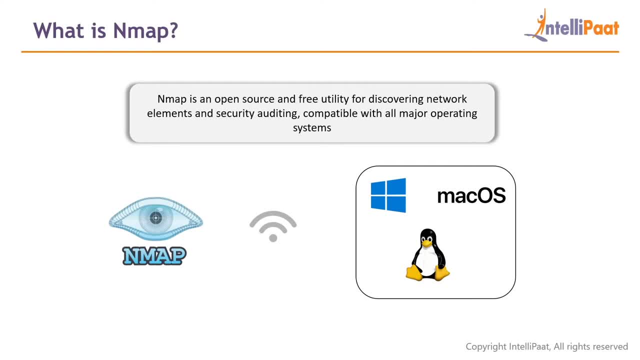 How many devices are connected. If there are any strange devices that are connected, if you're a hacker, if you're an ethical hacker or an hacker, you can use it to discover hosts on the target network as well. So that is the function of the NMAP application, right? 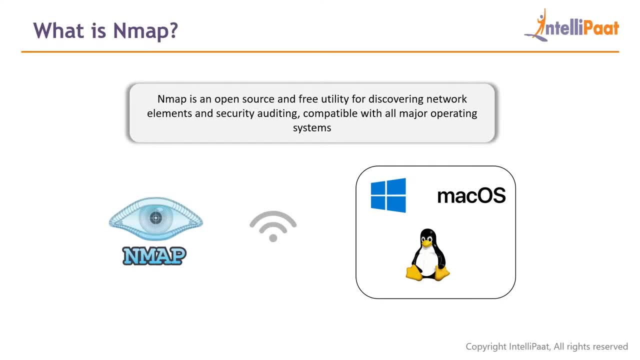 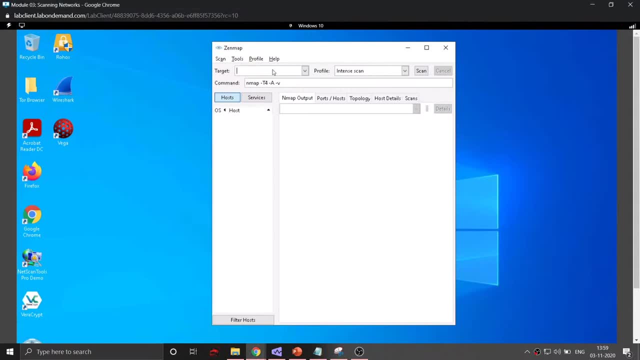 So we look into that as we move and proceed with the tutorial. So currently I have my NMAP GUI open. So firstly, uh, we're going to understand how we can detect all of the ports, uh, all of the services that might be open, or to confirm whether a particular host exists on a network or not. 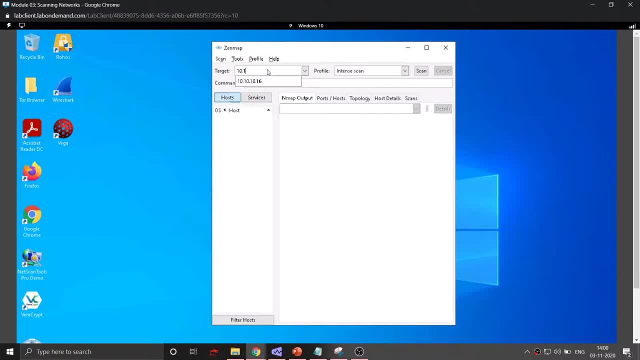 So, firstly, I'll ping a particular IP which is of the Windows Server 2016.. So I'll ping this IP by typing the IP address in the local network and I'll write the NMAP command that I want. So, in this particular case, I'll write SN and capital: PU, right. 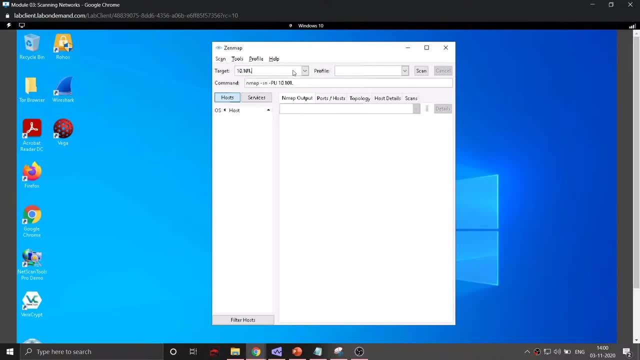 And then I'll put in the IP address again. I think I'll put it over here again and then put it over there, right? So when I click on scan, it'll first check whether the host is there or not And then, as we can see, it also says, after scanning the network, whether the host is up or not, and we can see that it is up. 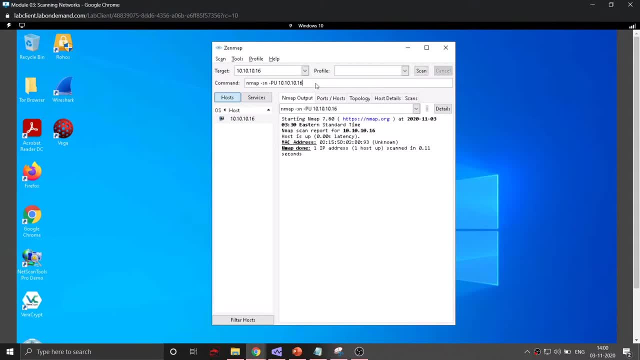 Right. So next up, uh, we can do something else with it. Uh, we can convert this particular into an ICMP echo ping scan. So by doing uh PE instead of PU, we can uh initiate that as well. 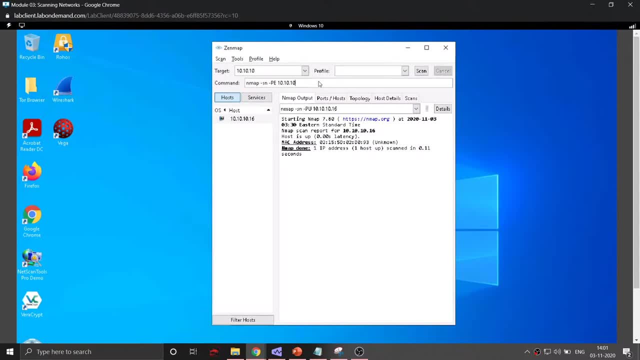 So 10.10.10.16, we type that and we click on scan, So it does that. And this is another way to basically detect If uh any particular host, uh with a particular IP address of that sort exists or not. 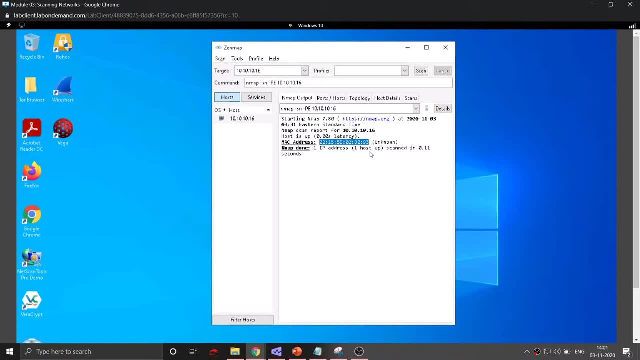 We can also see the Mac address for this particular IP address, Then the next thing that we can do is, If we want to detect all of the IP addresses that are present within a particular range on a network, we can simply type the starting uh uh- parameter of the range and then 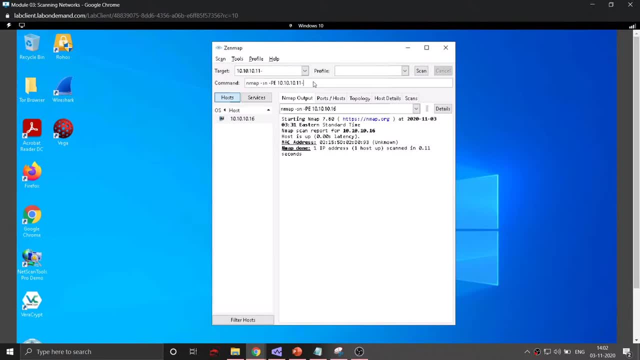 We can give a dash And then we can type the end parameter of the range and click on scan. So when we do that we can see all of the hosts that are present within that range. So if any intruder exists within that range, uh, in our particular network we are, we will be able to spot that particular intruder. 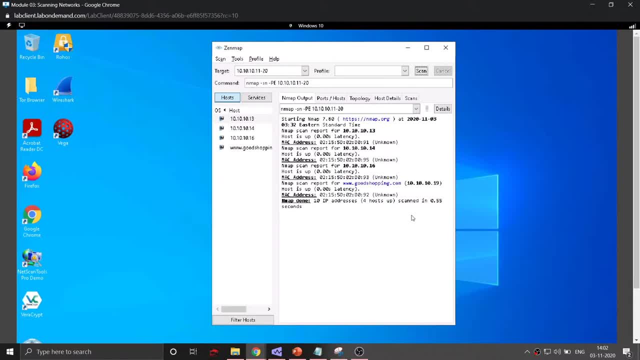 So we can see that Nmap will help us with a network security, with the various options and commands that it has Uh, especially when we are trying to track down And if if any particular suspicious activity is uh present on the network or not. 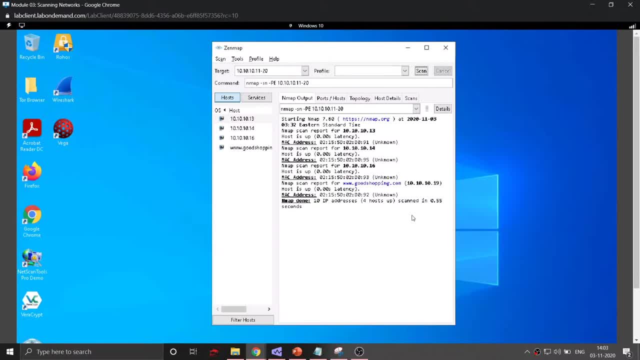 if any suspicious host is present on the network or not or if there are any security vulnerabilities on the system. So if Any of those exist, we can simply see it over here in the Nmap application and go fix them so that they don't exist anymore. 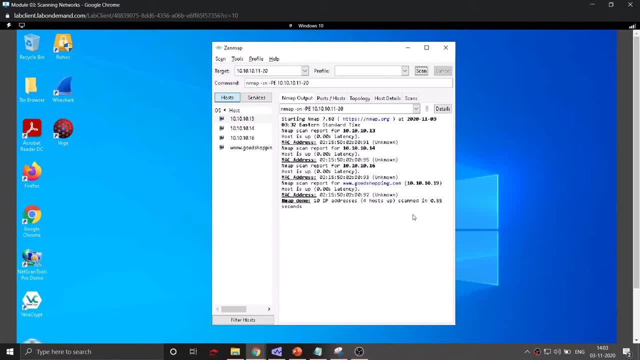 So this was it for the Nmap tutorial. We can see how well we can a a provide network security with the help of nmap. there are a lot of other applications as well that lie in the cyber security domain to help us with network security, such as wireshark and. 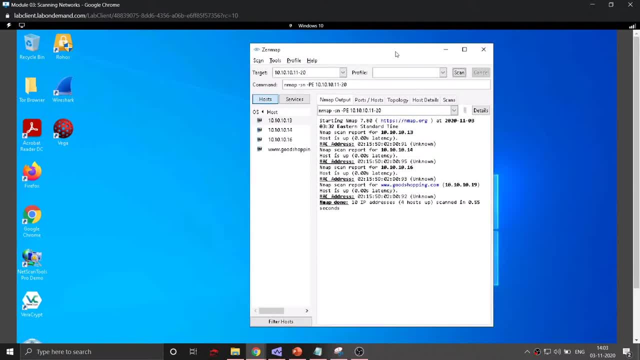 netscan as examples, right. so if you go ahead with the cyber security course, or any course with that matter, you'll be introduced to these applications as well and see how they implement network security on a network and how they can be used for ethical hacking as well. and 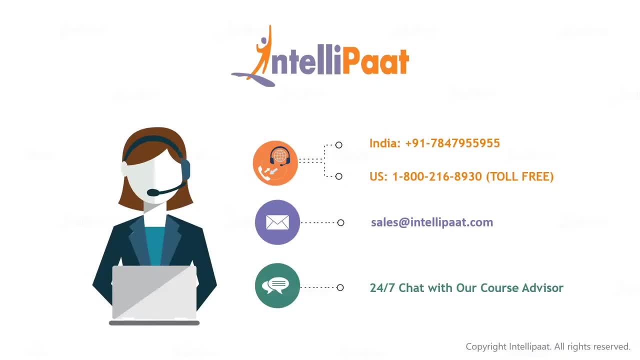 preventing hacking as well. if you've liked what you've seen, you can apply for one of our courses in the cyber security domain, where we cover cryptography and other such topics relevant to ethical hacking for our ceh certification training. you can contact our course advisors using the following contact details. they are available 24: 7.. you can also mail our sales team. 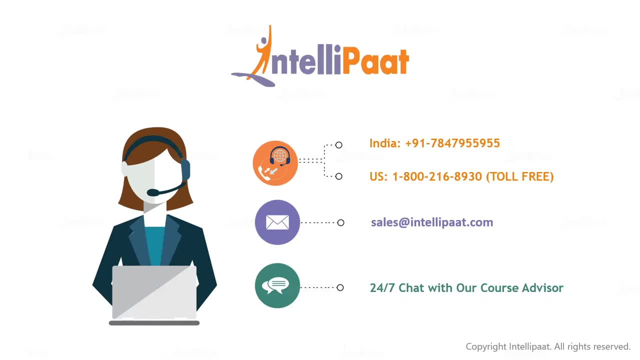 to inquire about any of our courses or have a live chat with our course advisors on our website, intellipaatcom. so, uh, one another thing: be sure to sign up for our webinar. we post videos like these daily. we host webinars like this daily, so be sure you sign up for that and not miss out on any content from us and actually have the 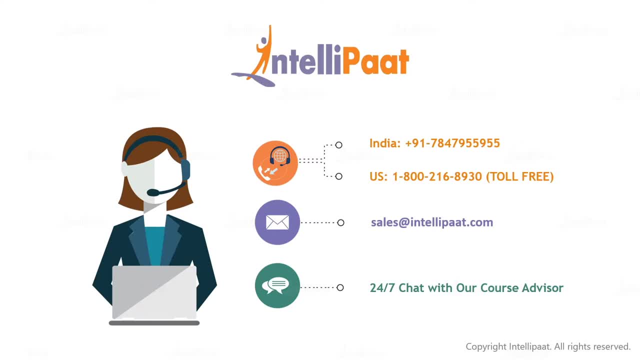 ability to ask us live doubts if you sign up for the webinars and attend our meetings. right? so that is about it from intellipaatcom. hope you had a wonderful session. be sure to like this video and subscribe to this channel if you've liked what you've seen. thank you and goodbye. you.